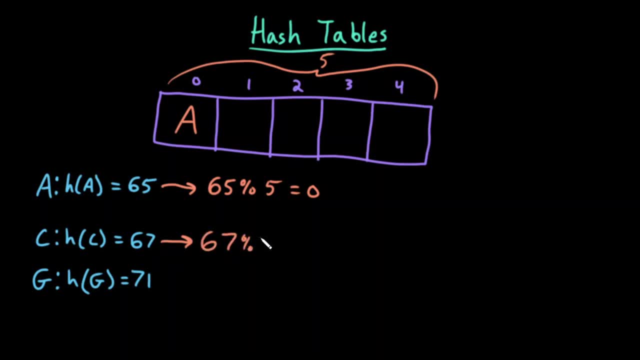 mod it by the length of the array, which returns 2.. So the index of C will be index 2.. Let's try one more example. The hash value of the letter G is 71, which then modded by 5,. 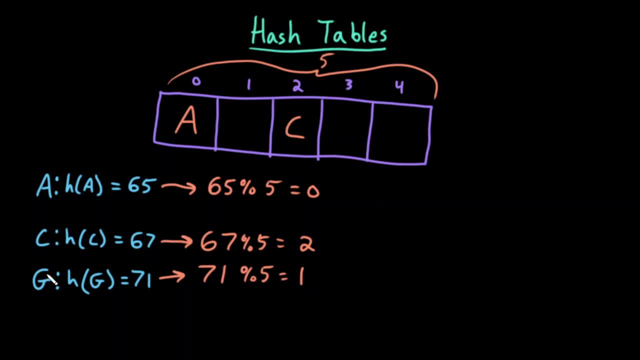 to get an index in this array is 1.. So G will be inserted at index 1.. Notice that I picked numbers that would not overlap in terms of their indices For this specific video. we're going to assume that we never have overlaps. 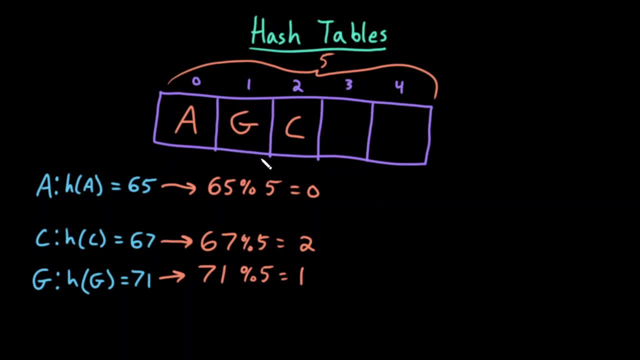 aka collisions, And in a future video we'll discuss what do we actually do if two different objects map to the same exact index. But for now, don't worry about it. So that was the insert algorithm. It was super simple. We just hash our element. 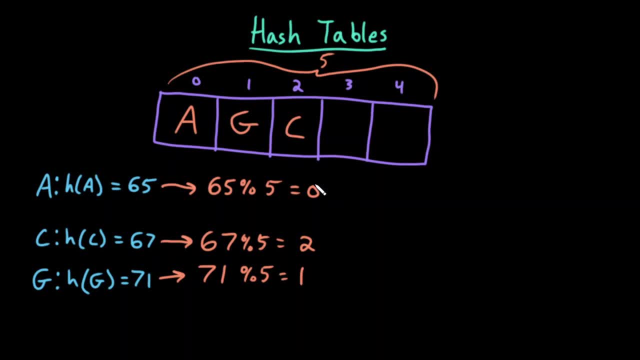 mod by the length of the array and that gives us an index. How do I check if an element exists? So what if I asked: does the element C exist in this hash table? Again, I would just hash my element. So I would hash C. 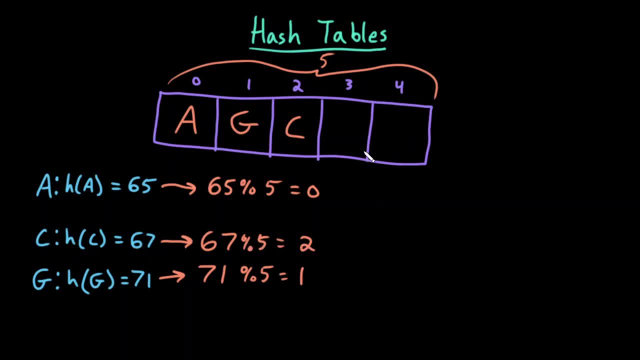 I would then mod it by the length of my array And then I would check: oh, it does exist. C is at this index. What about if I wanted to see if the element D exists in my array? So the hash value of D in my simple hashing is just going to be the ASCII value. 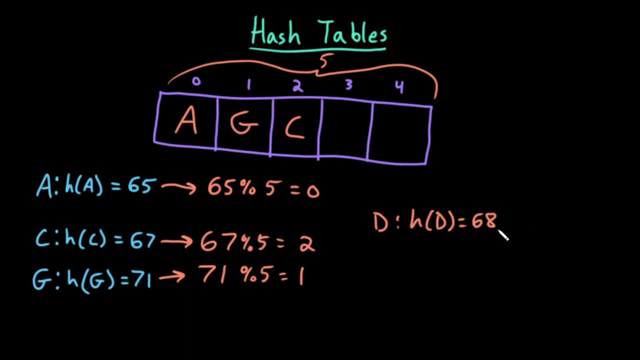 So the ASCII value of D is 68. And then to get an index, I mod it by the length of my array, which gives me 3.. D existed in this hash table. it would appear at index three. So I jumped to index three and I see. 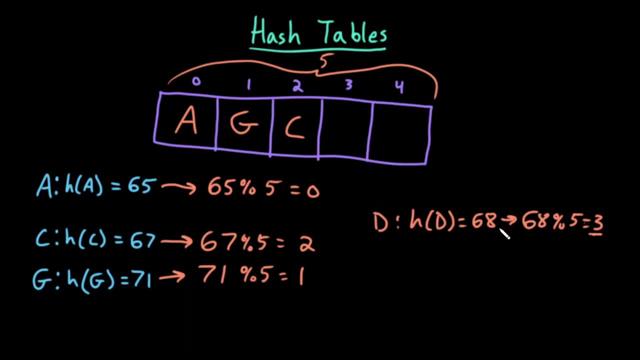 no, D does not exist here. Therefore, D does not exist in my hash table. Let's try one more example. What about if I wanted to find the letter F? So the hash value of F, the hash code of F, is the ASCII value of F. 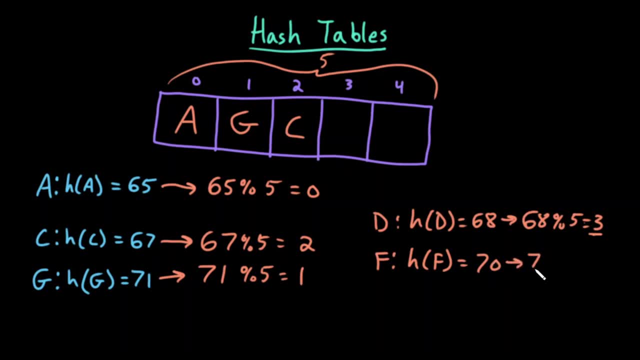 which is 70.. And then to convert that into an index, 70 mod by the length of my array is zero. I jumped to index zero And even though index zero is not empty, it doesn't contain F. Therefore, under this simple example, 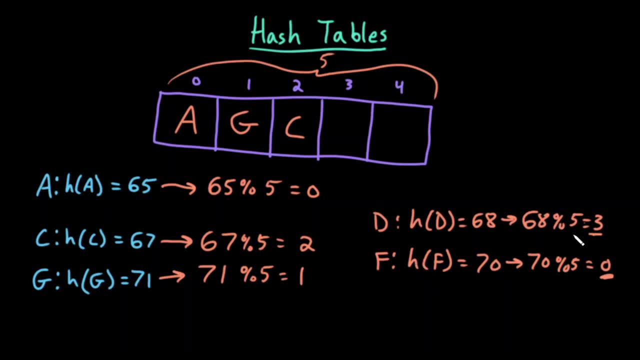 where I'm not taking into account potential collisions, I would say F does not exist because F is not in this index. If I were to remove an element- let's say I wanna remove the element C- again I get the hash value. 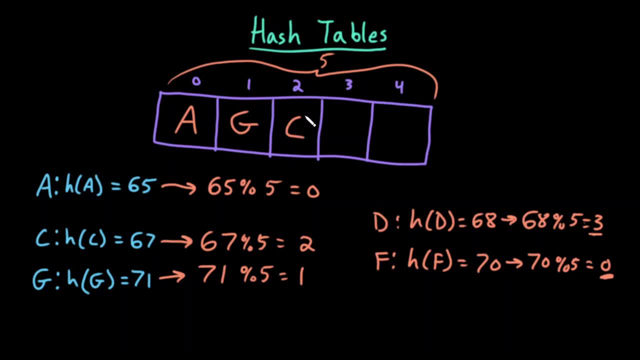 mod it by the length of the array. that gets me index two and then I would just remove it from that index. So find, remove and insert are extremely trivial, if I ignore the fact that collisions can happen. If you think about it, the hash table implements: 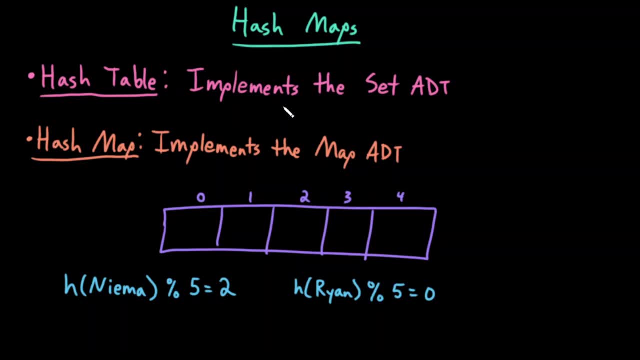 the set abstract data type: A hash table. for a hash table, I can insert elements, I can check if a given element exists and I can remove elements. which exactly describes the set ADT. The hash map is a slight extension of the hash table. 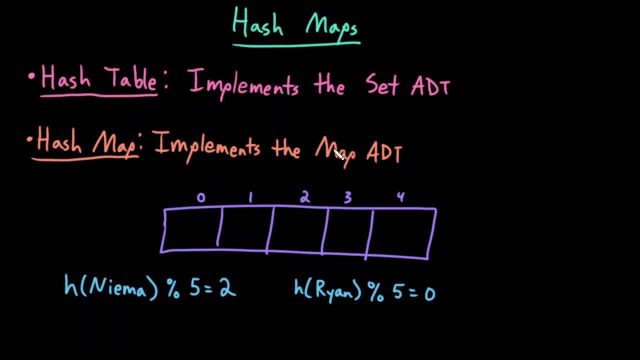 but which implements the map ADT. So instead of inserting individual elements in a map, like a hash map, I insert key value pairs. So I insert a key with its corresponding value and I insert a key with its corresponding value, and instead of retrieving 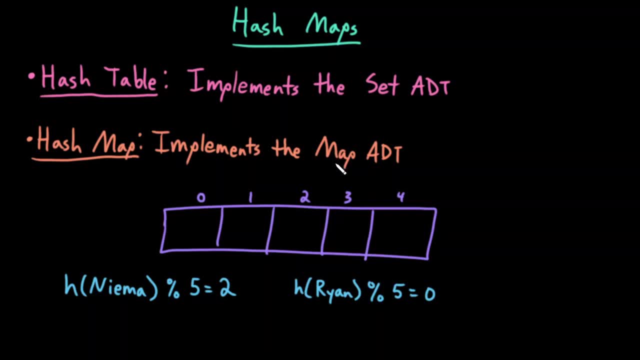 instead of just checking if an element exists, I can retrieve the value associated with the given key, And likewise I can remove a key value pair if you gave me the key. So in this example, again, just like a hash table, a hash map has some array behind the scenes. 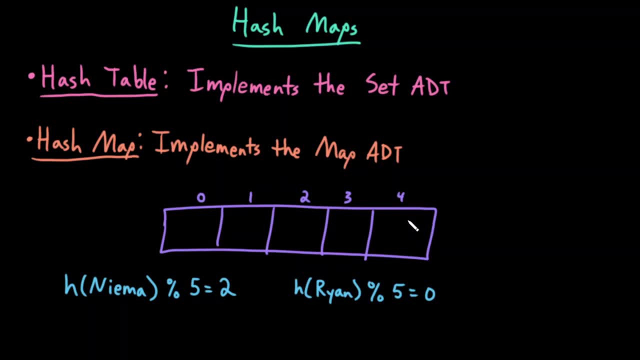 I've drawn one that has five empty slots. This hash map doesn't contain anything. And let's say it's a hash map that will map strings to strings. Let's say I wanna map student names to student grades. I've written down two student names: Nima and Ryan. 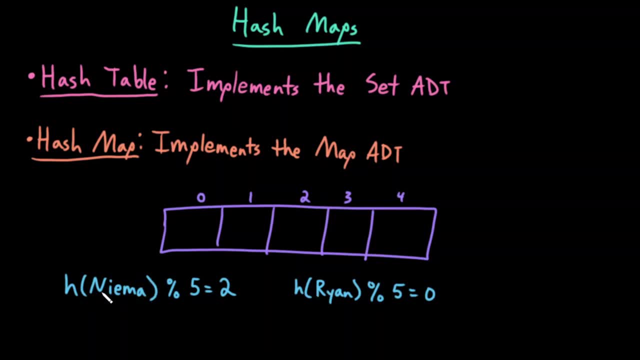 and I don't feel like getting into the details of whatever their hash values might be, but let's just say that whatever their hash value is, mod five will return two for Nima And let's say the hash value of Ryan, whatever it may be. 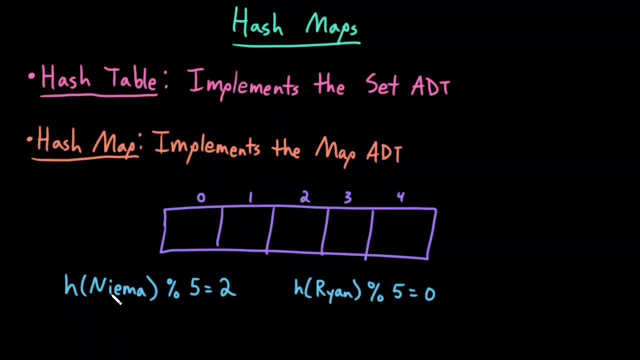 mod five is zero. Remember, given the hash value of a given object, if I mod by the length of the backing array, that gives me the index that that object should appear. So Nima should appear at index two. Ryan should appear at index zero. 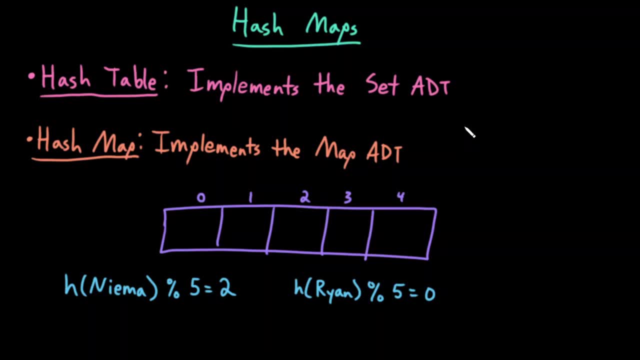 So let's say I wanna add the key value pair whoops Nima A plus. So I wanna give Nima a grade of A plus. Well, with respect to the key, I have to add a grade of A plus. 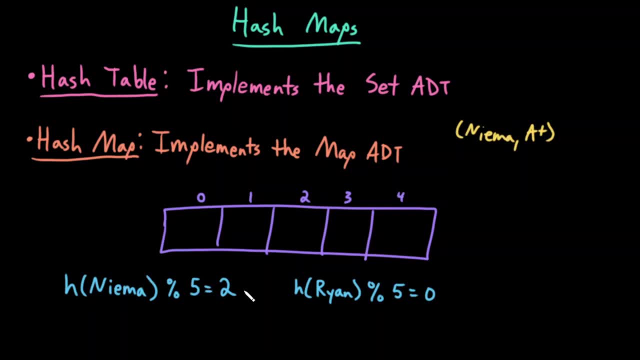 Well, with respect to the key, I have to add a grade of A plus. I hash it and mod by the length of the array to get an index, which is two, and I will insert this key value pair: Nima A plus. 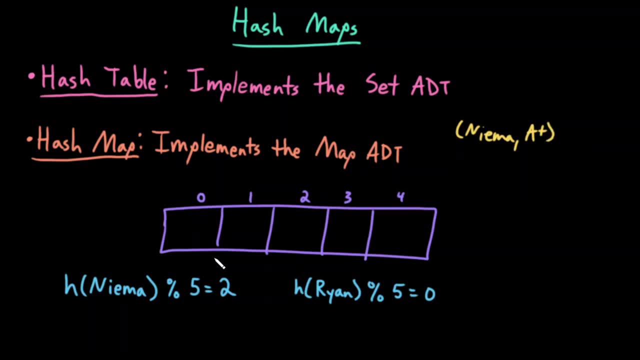 oops, index two. sorry, Nima maps to index two, so I will add Nima A plus to that corresponding index. Let's say I wanna add Ryan, let's call it index two and I will how a string A to my hash map. 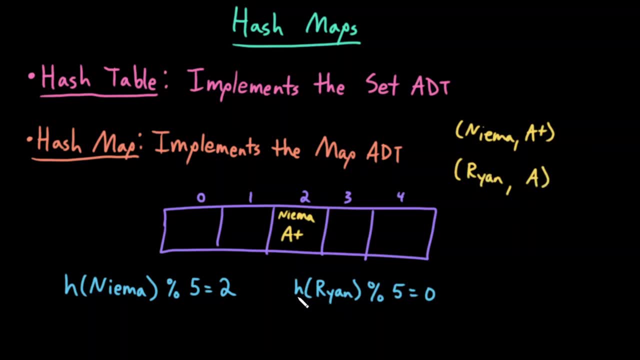 So I wanna map. so I want Ryan to have a grade of A. I would hash the string, Ryan mod it by five to get an index in this array and it returned zero. this time I'm doing it right And I'm gonna insert that key value pair into index zero. 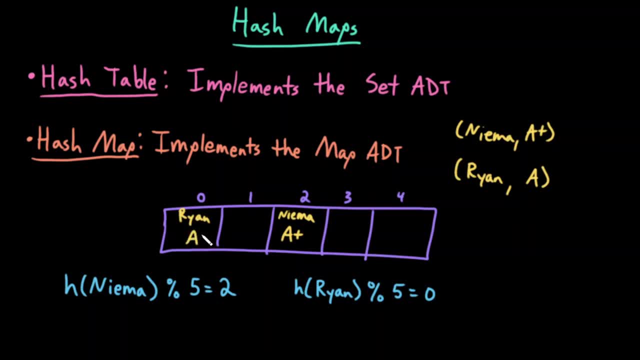 So the key is Ryan, the value is A. That was the insert function of a map. I can then retrieve the grade. Let's say I wanted to know what is the grade of Nima. Well, again, I would mod Nima by five. 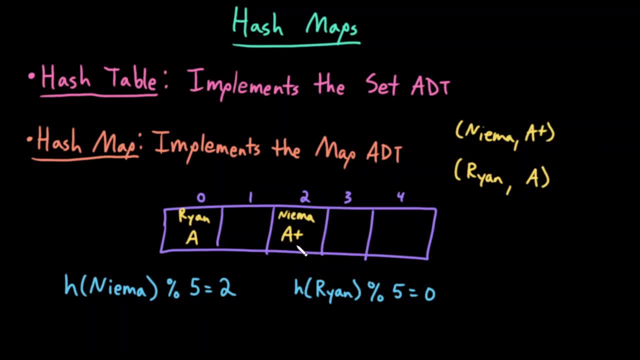 go to its index, which is two, and I would say, oh, the value associated with that key is an A plus. If I wanted the grade of Ryan, so retrieve the grade of Ryan. I will, hash Ryan, mod it by the length of my array.